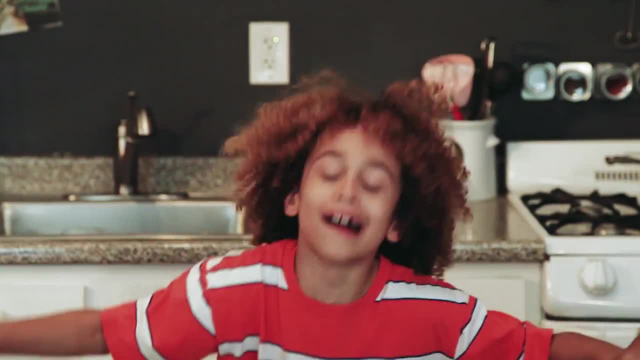 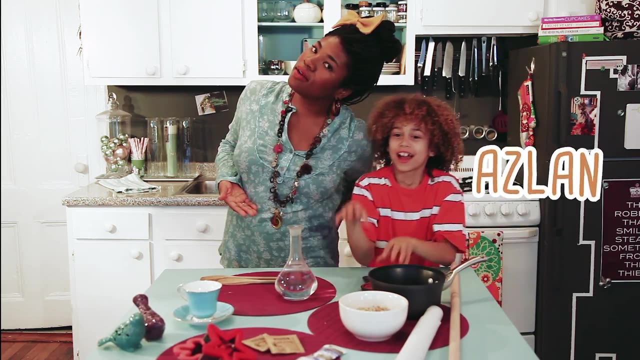 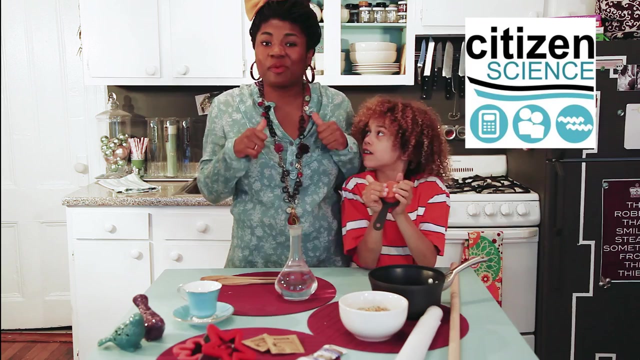 Hey everybody. it's Chrissy, Aunt Lindsey and you are in the Fab Lab. I'm here with my Fab Lab professor, Aslyn, Say hello, Hi. And today is super, super special. I am going to be announcing my Citizen Science project for the season. 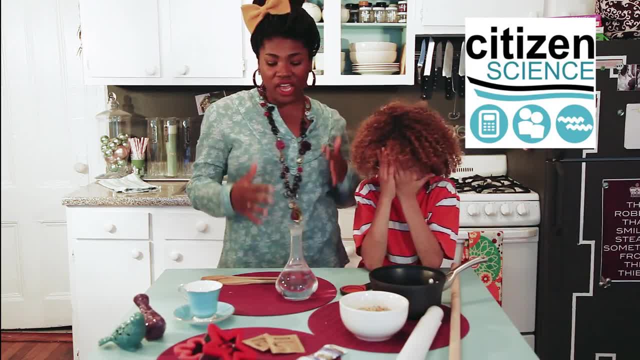 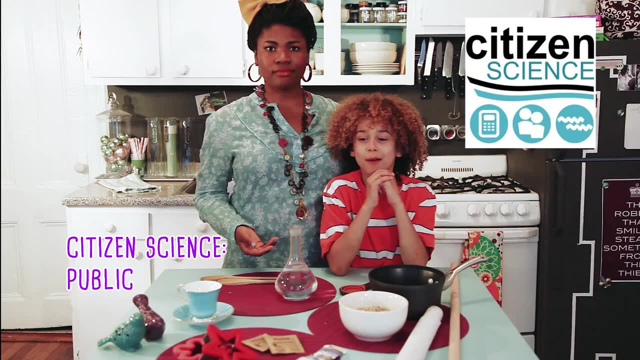 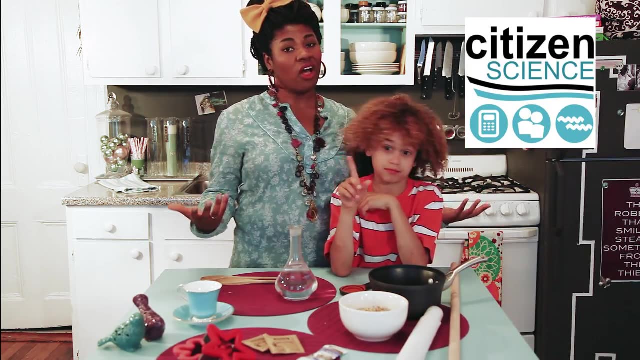 And then, in honor of that, we are going to do a very special project to celebrate. So, Citizen Science- what is that? Citizen Science is a public participation in science, research. Well, that's funny, because some people seem to think that the only people that get to participate in scientific research are people wearing lab coats and have PhDs. 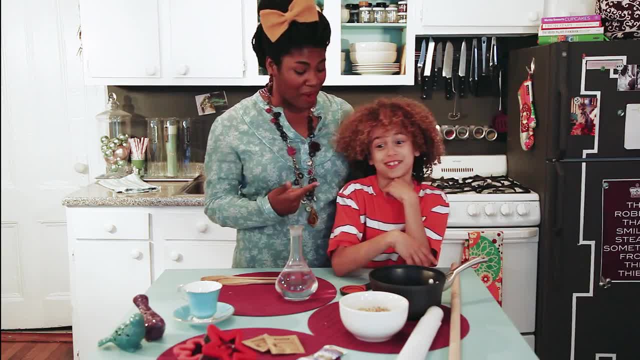 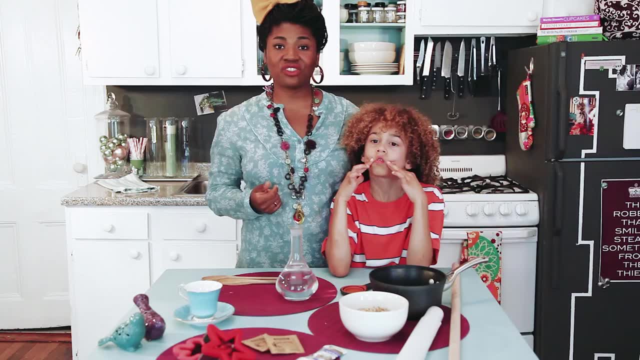 That's not true. It's not true. You're absolutely right, Aslyn. Thank you for telling us, Because the truth is that people all over the world are conducting high impact scientific research all over the globe. NASA even has a Citizen Science program. 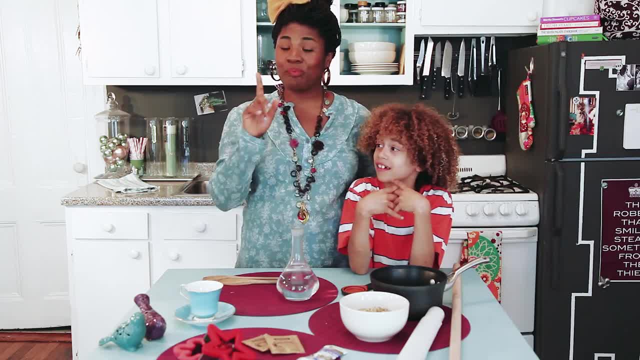 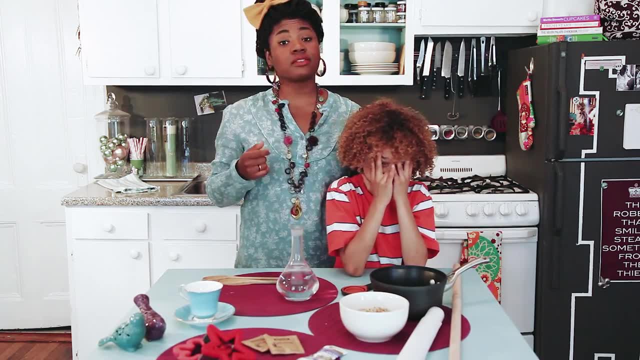 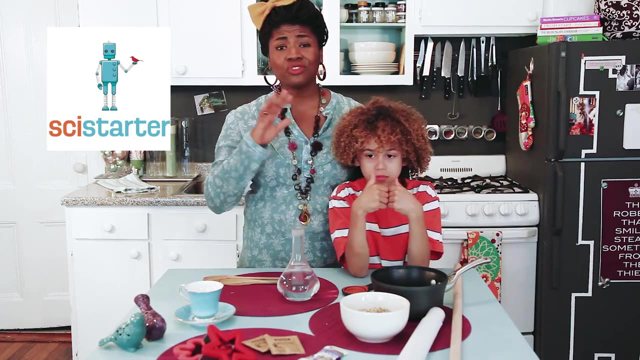 Now. I won't be going into space anytime soon, but I am going to be doing a Citizen Science project right here in my very own backyard. I recently discovered SciStarterorg, which is the database for Citizen Science projects. You can go there and do a search for all sorts of projects happening in your neighborhood over all sorts of interests. 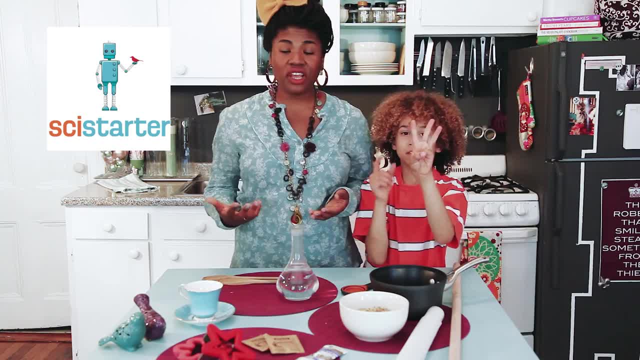 I mean, there's stuff there for astronomy, biology, watersheds, I mean you name it. I didn't know there were so many Citizen Science projects happening across the globe, But now that I know that I'm going to do it. 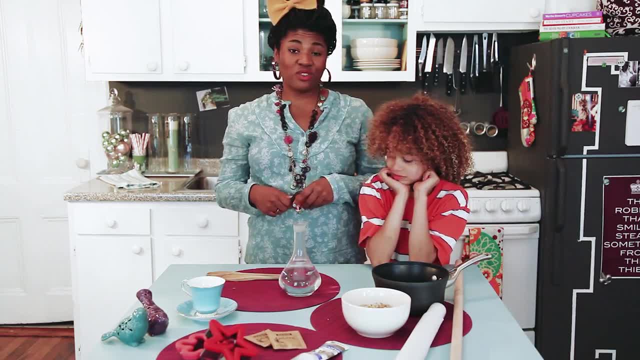 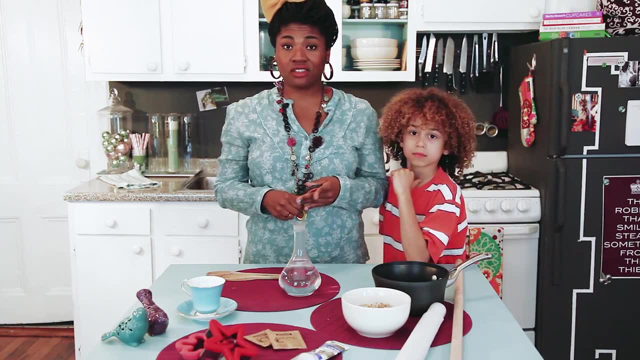 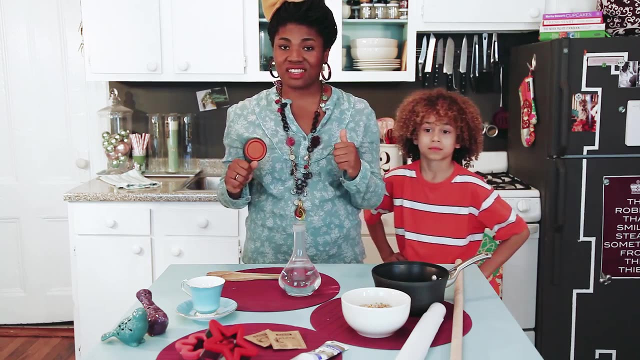 And what I do. I am hooked. So I'm going to be using SciStarterorg to choose one project every few months for my Citizen Science exploration. So that brings us to some very, very important news. My Citizen Science project this season will be: 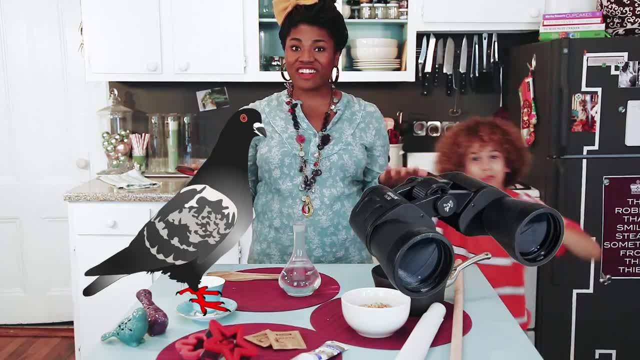 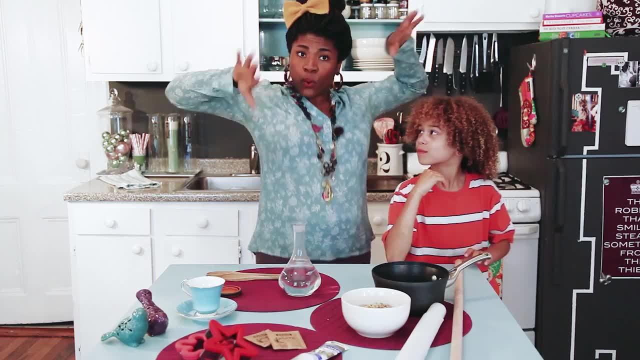 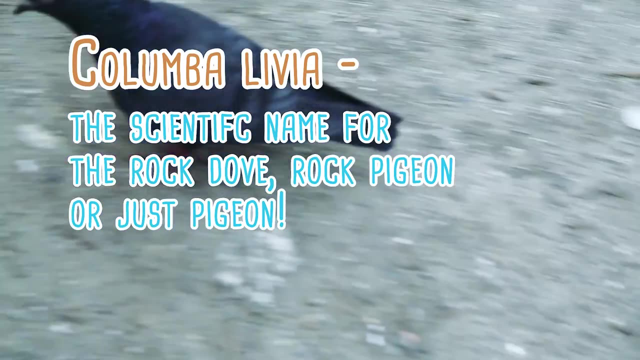 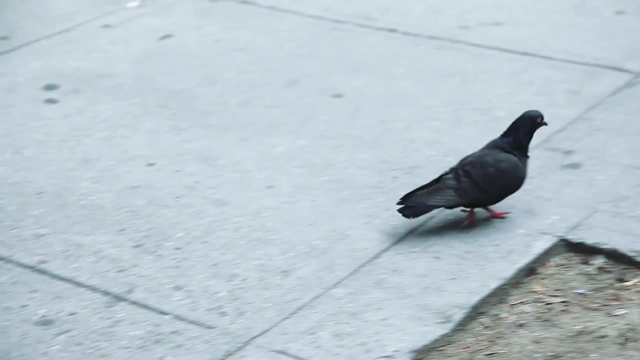 Bitch The Pigeon, Watch Fine, No, Okay, New York City's mascot bird, the Columbolivia or Go pigeon Are curious little creatures. They are mainly city dwellers. They don't migrate And their mating habits are pretty peculiar at times. 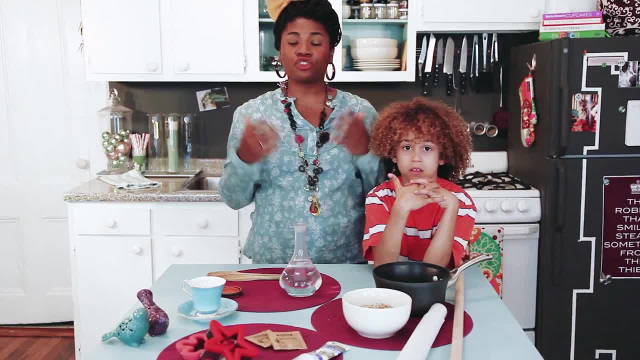 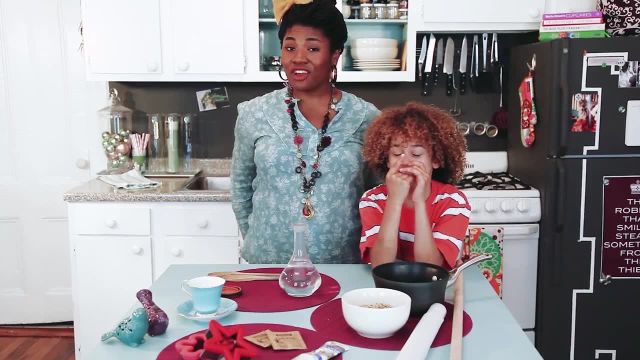 So I will be helping the Cornell Lab of Ornithology track their courting behavior for the next few months, And in honor of this project announcement, we are going to show you how to make not one, but TWO bird feeders. 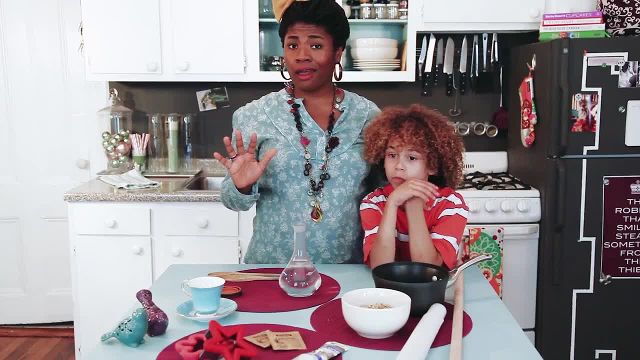 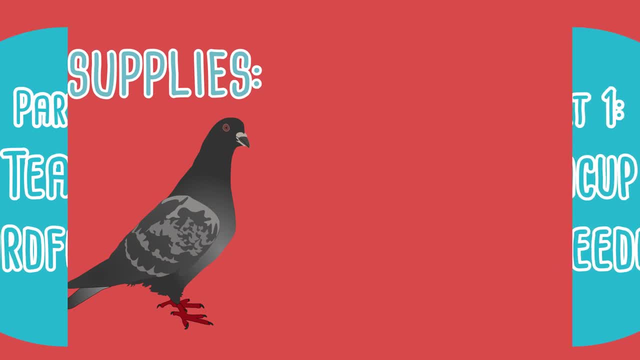 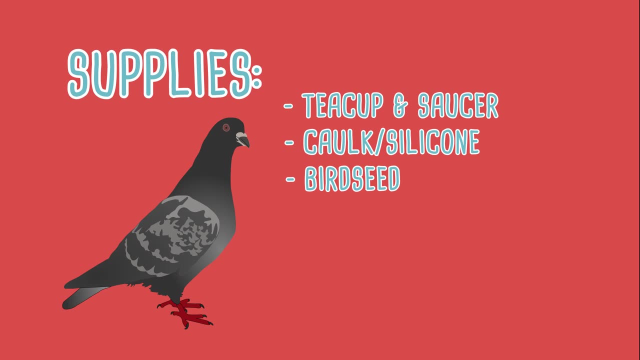 Oh yeah, And these are not just any bird feeders, people. They are Fab Lab-lucious. For the first project, all you're going to need is a teacup and saucer, caulk and birdseed. Now, this one is really really simple. 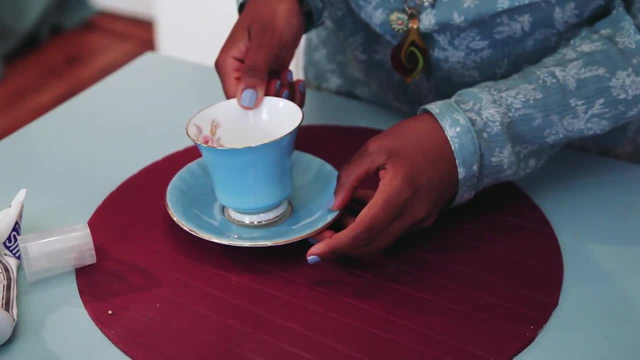 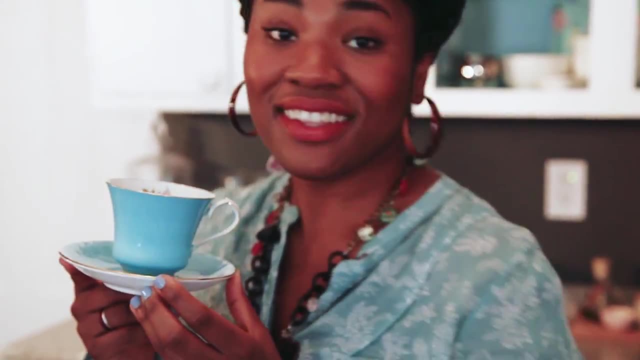 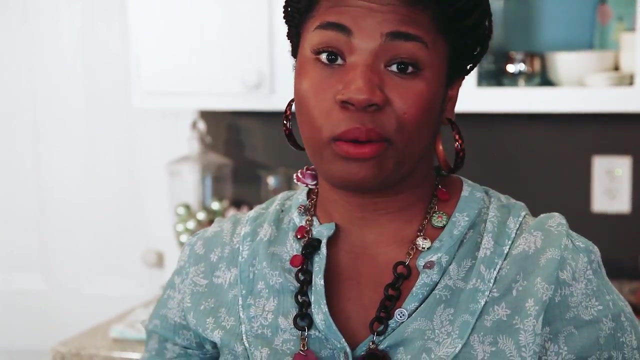 All you're going to do is take your teacup, line it with a little caulk and then stick it onto the saucer And let it dry. Make sure you're paying attention to the drying instructions on the packaging. This one is just three hours, but some caulk can take up to 24 hours to dry. 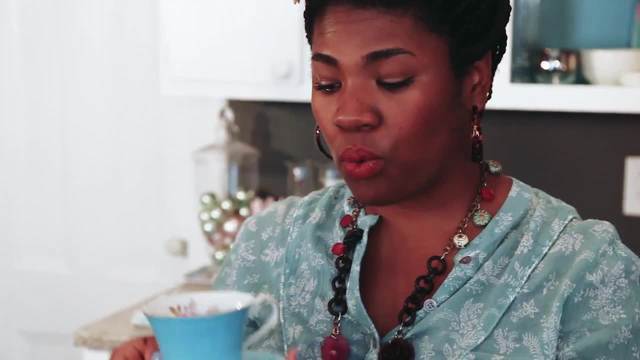 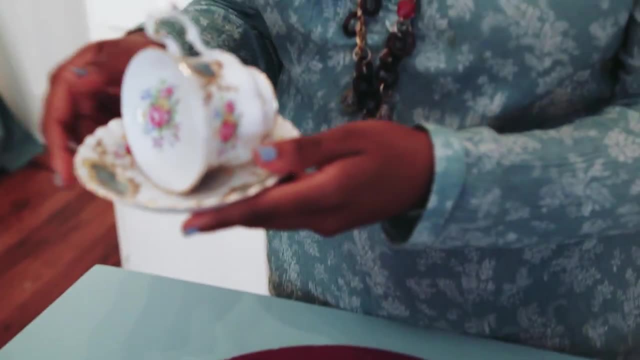 So make sure you look at the package for drying instructions. Now we're going to just set this one aside to dry, but we pre-made one. And look at how fancy this one is. I love that Aunt Michelle glued it on an angle. 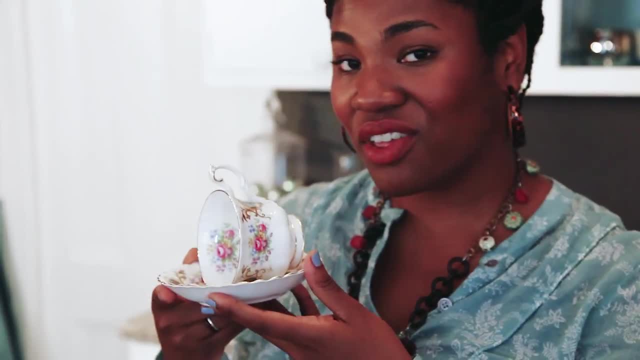 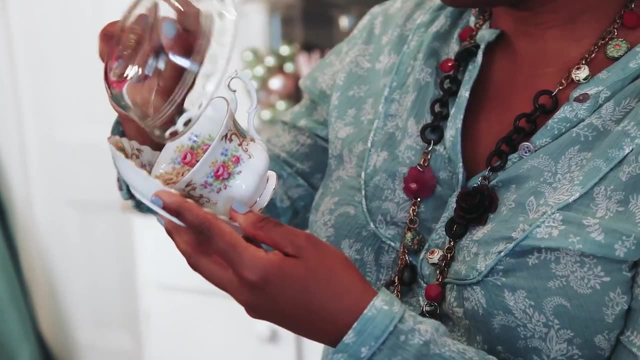 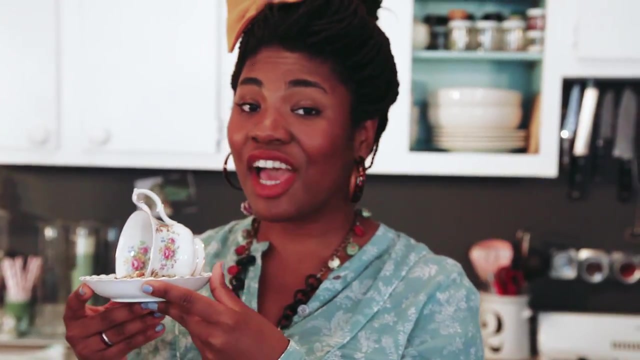 Ah, it's so pretty, So we're going to- We're going to fill this with our birdseed- Really easy, Like this- And then let it spill out just a little bit Beautiful. Now you're ready to take this outside and set it in your family's beautiful garden. 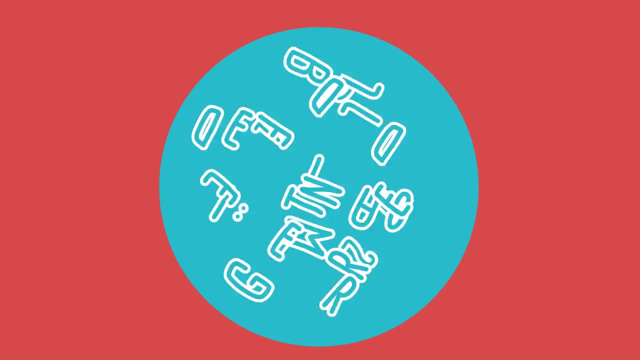 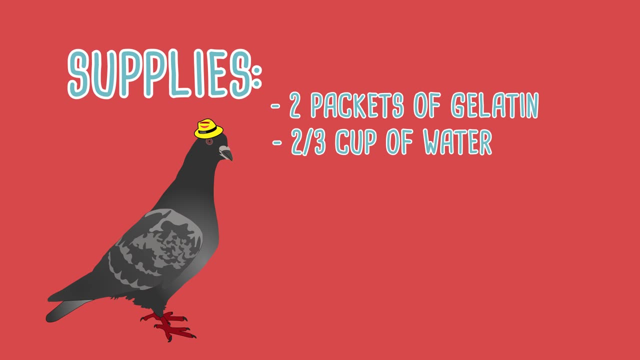 and watch the birds flock to this buffet. So for this portion of the project, you're going to need two packets of gelatin, two-thirds cup of water, two cups of birdseed parchment or wax, paper, straw, twine. 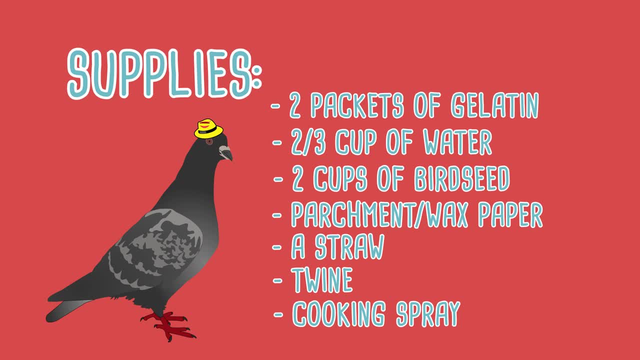 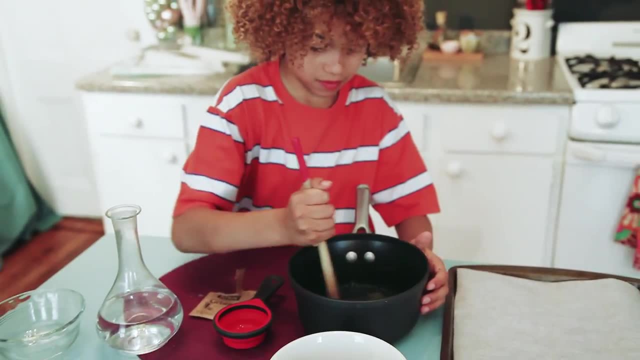 and a little cooking spray for your cookie cutters or molds. So the first thing you're going to do is dissolve your two packets of gelatin and your two-thirds cup of water in a pot. Now have an adult stir this over medium heat over the stove. 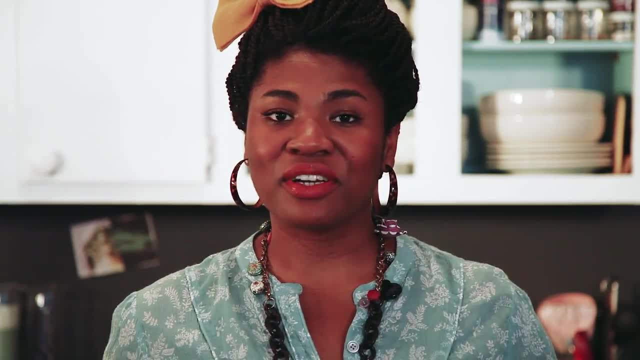 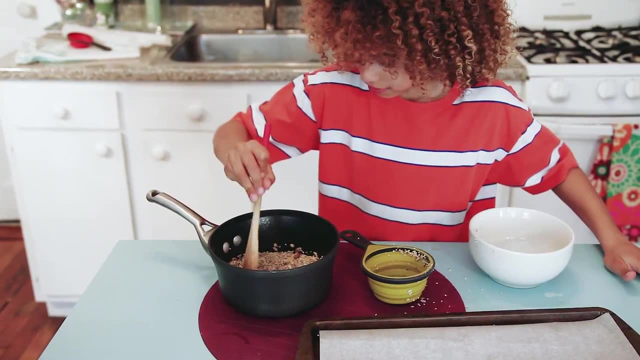 for a few minutes until it's simmering. Now, once it simmers, I want you to remove it from the heat and let it cool off for a little while. Throw in the birdseed, Mix it up. Now spray your molds with the cooking spray. 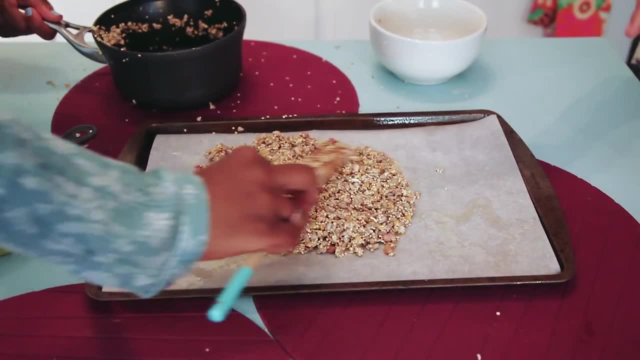 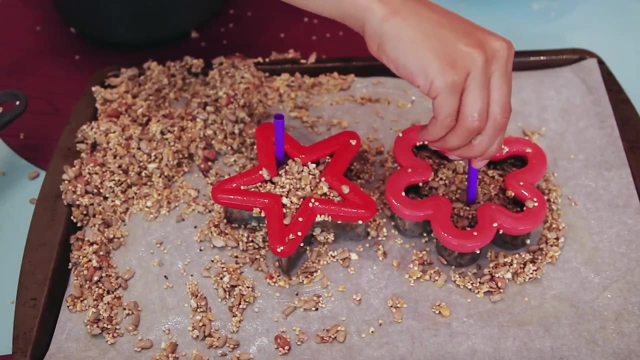 and then spread it over parchment paper lining a cookie sheet And then fill them up with your birdseed gelatin mixture. Now use a straw to punch a hole in the top of each of them and then toss them into the refrigerator so that they can set for about an hour. 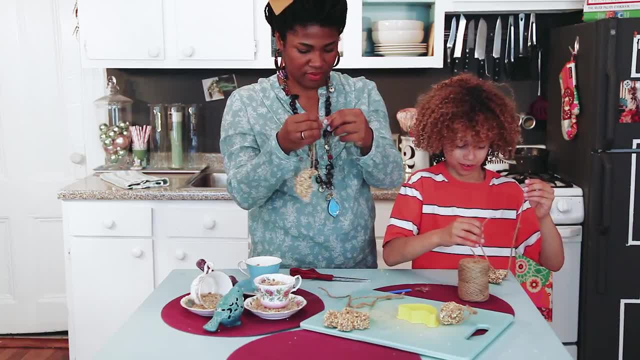 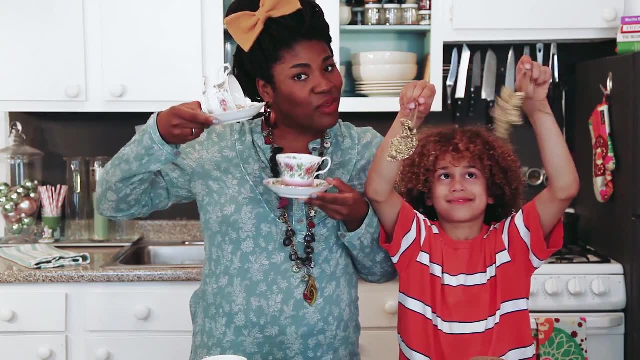 Now take them out of the refrigerator, string them with twine and go hang them outside on a tree or on your city balcony. Alrighty, here are our beautiful bird feeders. We are going to set these outside and keep our eye out for those pigeons. 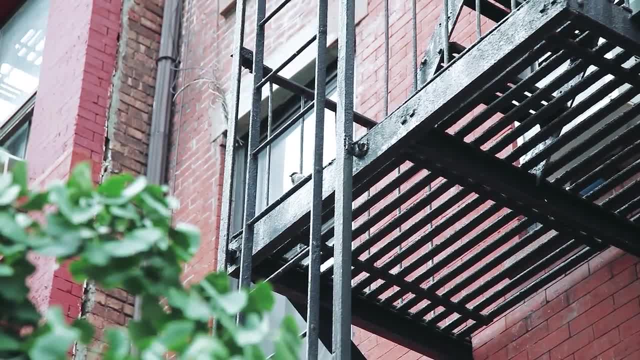 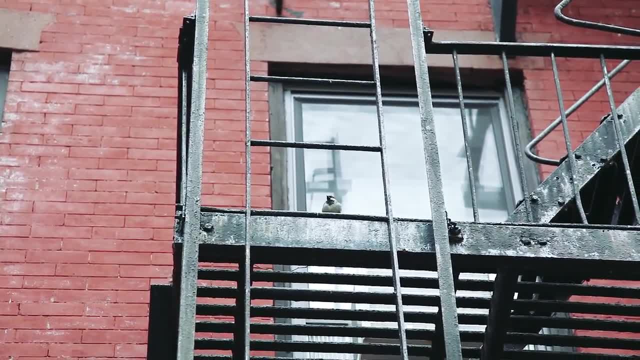 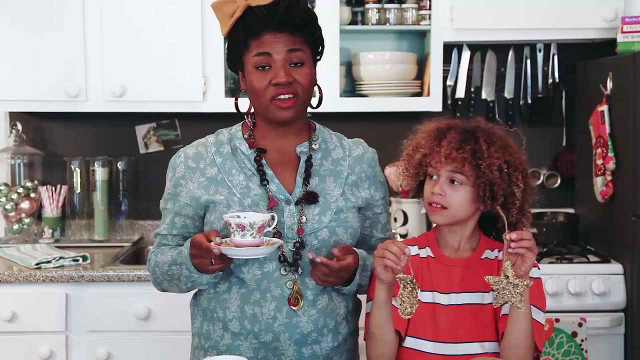 But what birds are native in your neck of the woods? I want you to do a quick search at scistarterorg and let me know what birdwatching activities they have going on in your neighborhood that get your birds chirping. Leave a comment below with the link to the project that you plan on looking into. 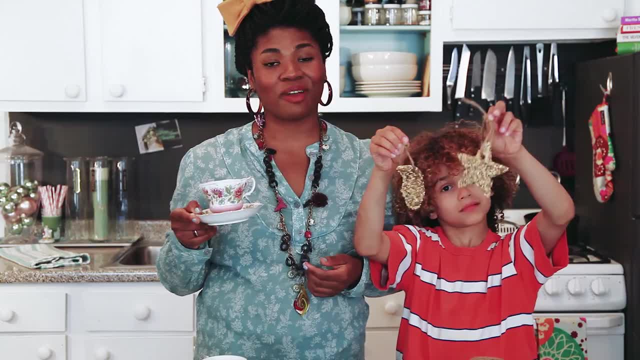 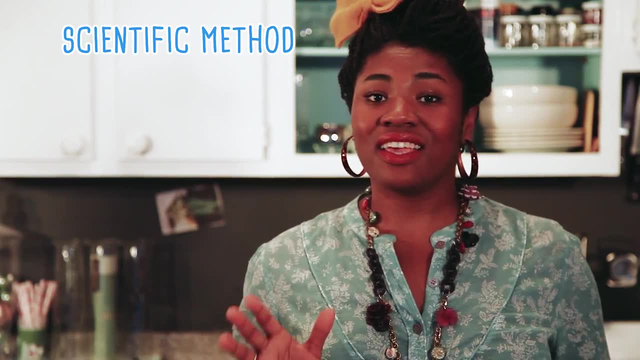 I would love to see what you guys have going on in your citizen science projects. This episode is a study in life science and habitat. Now there are five basic steps in scientific method: Observation, hypothesis, experiment, data collecting and reporting. 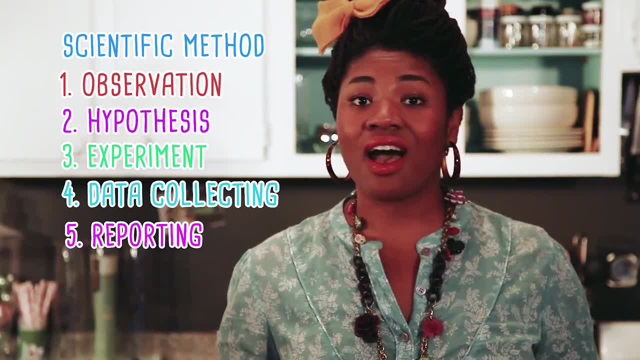 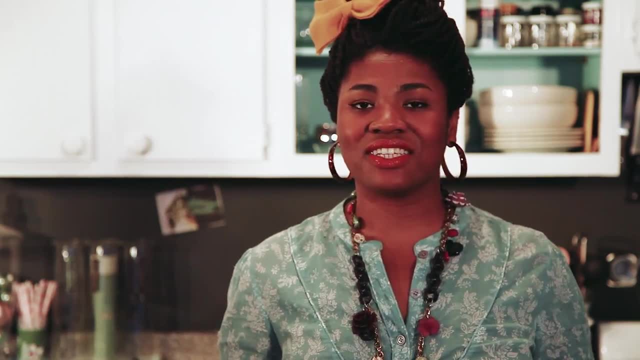 This project focuses on three of those five steps: Observation, data collecting and reporting. Now, over the next few months, we're going to be observing our little friend pigeons and then collecting data about our observation. Then we're going to report back to the Cornell Lab of Ornithology. 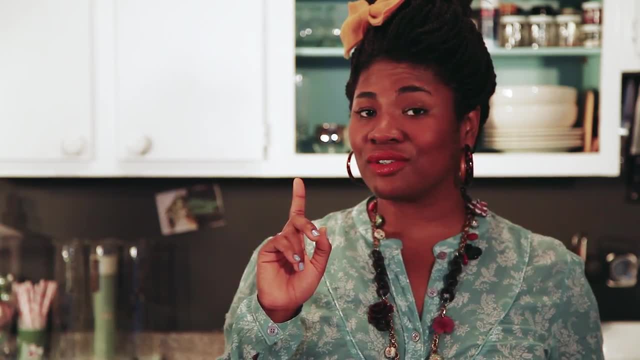 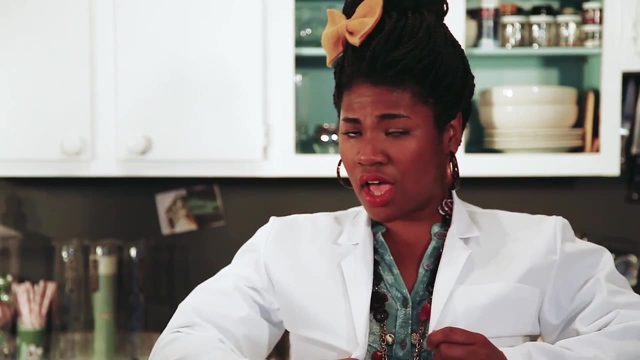 on our findings. And not only that, but we're going to use our beautiful bird feeders to attract our specimens for this wonderful experiment. My lab coat is on and my safety goggles are here, Not on my face. That can only mean one thing. 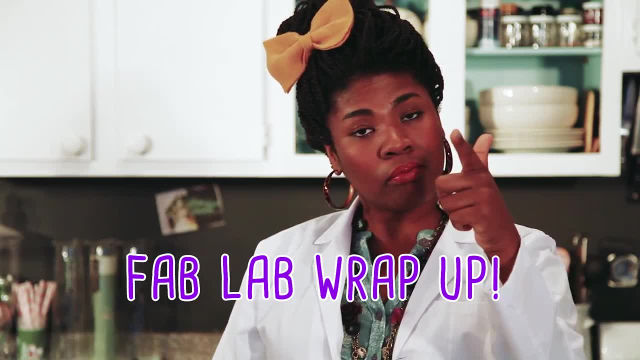 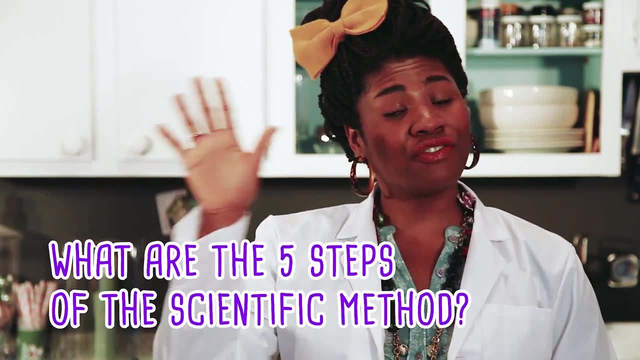 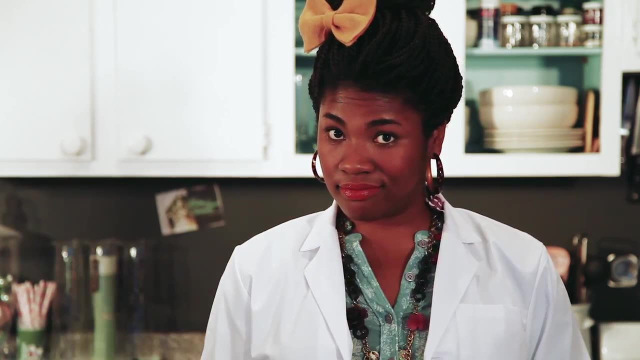 It's time for the Fab Lab Wrap Up. So I know that you have been paying attention to me And not the firetruck outside. What are the five steps to the scientific method? What is the scientific method? What is the scientific name for pigeon?